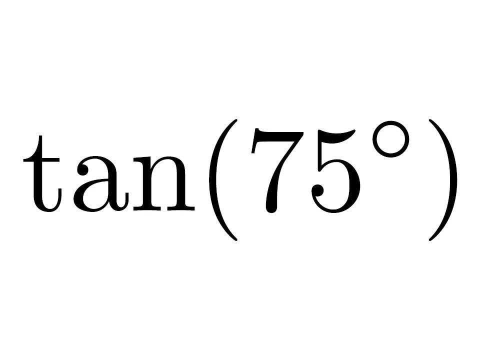 In this video we are going to find the value of 10 of 75 degree. The 75 degree is equal to 45 degree plus 30 degree. So 10 of 75 degree is equal to 10 of 45 degree plus 30 degree. 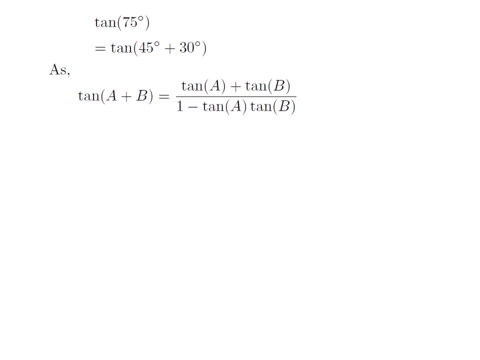 As we know, the expansion of 10 of A plus B is equal to 10 of A plus 10 of B, divided by 1 plus 10 of A into 10 of B. If you want to know how to derive this formula, the address of video is given in the description- Please check. 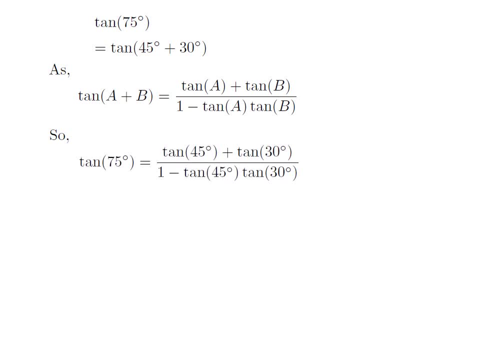 To find out the value of 10 of 75 degree, we just have to replace the 10 of A with 10 of 45 degree and 10 of B with 10 of 30 degree in the above formula. So 10 of 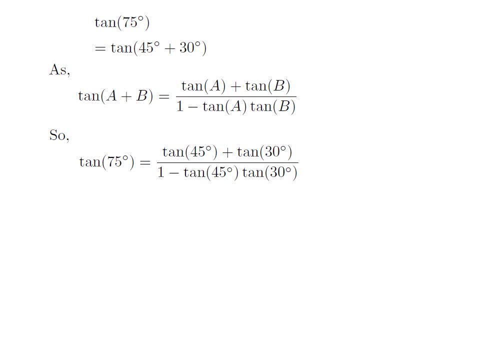 75 degree is equal to 10 of 45 degree plus 30 degree. So 10 of 75 degree is equal to 10 of 45 degree plus 10 of 30 degree, divided by 1 plus 10 of 45 degree. 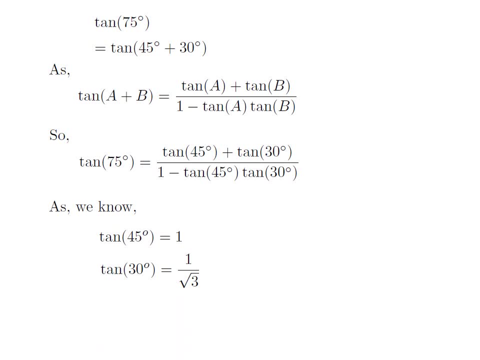 into 10 of 30 degree. As we know, 10 of 45 degree is equal to 1 and 10 of 30 degree is equal to 1 by square root 3.. So we replace these values in the above formula. So 10 of 75 degree is equal to 1 plus 1 divided by square root of 3 in. 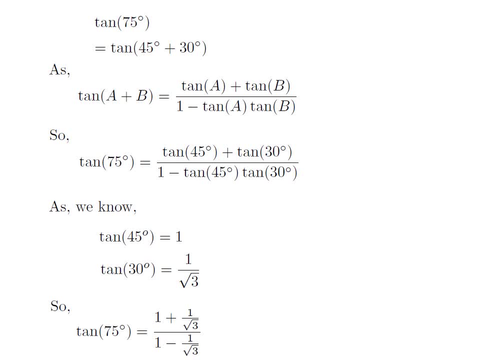 numerator and in denominator. So 10 of 75 degree is equal to 1 plus 1 divided by square root of 3.. So 10 of 75 degree is equal to 1 minus 1 into 1 divided by square. 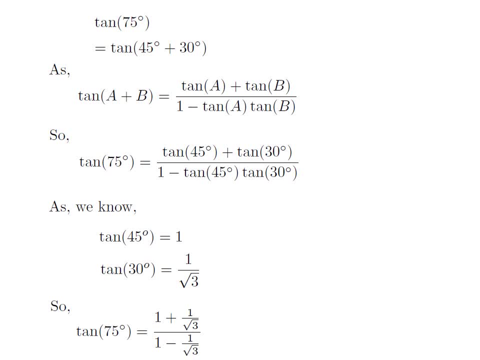 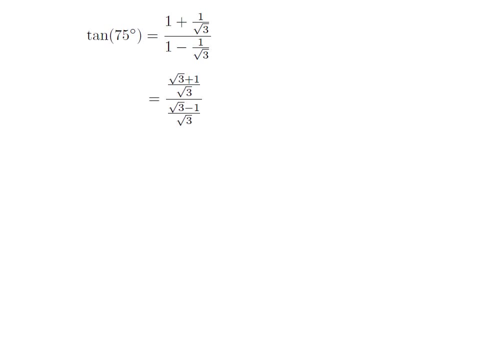 root of 3, which becomes 1 minus 1 by square root of 3.. Let's see the numerator expression Here. square root of 3 will be in the denominator, So in the numerator it will be 1 into square root of 3 plus 1, which is equal to. 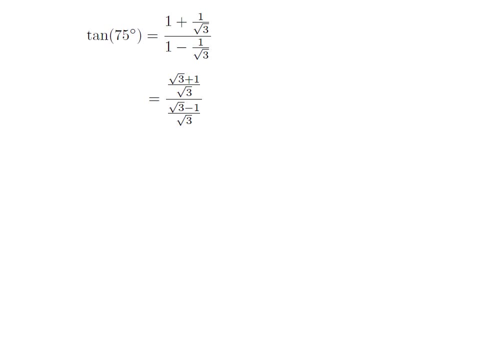 square root of 3 plus 1.. Same way, in denominator it is square root of 3 minus 1 divided by square root of 3.. Here I have further simplified it. The expression has become square root of 3 plus 1 divided by square root of 3 minus 1.. As multiplying the